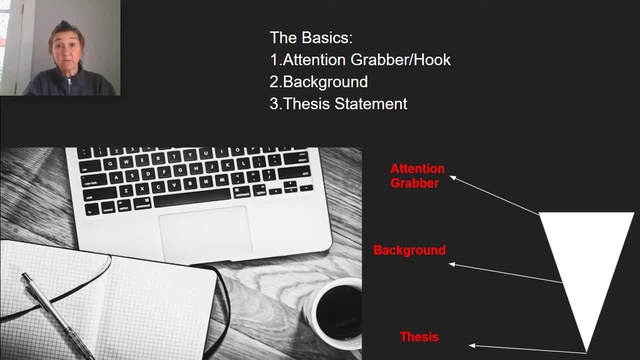 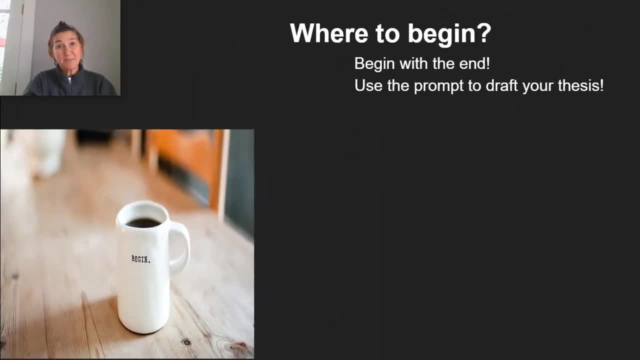 specific than the hook, and the thesis statement is going to be the most specific of all. So that's why that That visual works for a lot of students. So where do you begin? This is going to seem a little odd, but I think it's best to begin with the end in mind. So what I encourage my students 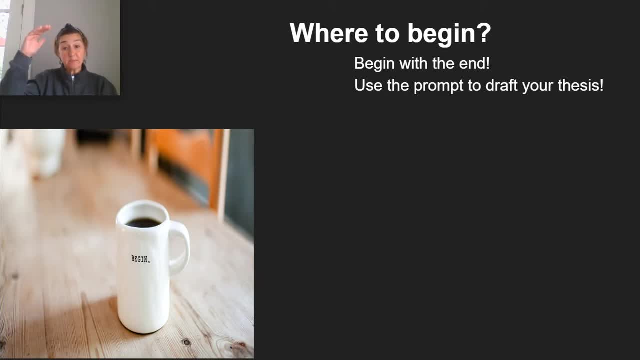 to do is to actually draft their thesis first. So I have them skip a few lines. draft their thesis first so they know where they're headed, and then they can go back and add the next steps. So let's take a look at a sample prompt. This might be a prompt you get in US history or English. 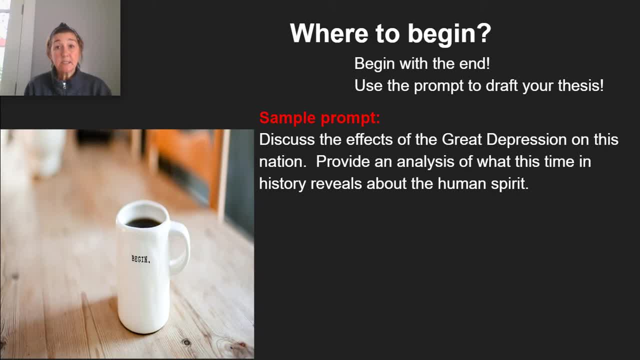 class, or maybe you're going to write a research paper, But this prompt says: discuss the effects of the Great Depression on this topic. So let's take a look at a sample prompt. So let's take a look at a sample prompt. So let's take a look at a sample prompt And notice I haven't said anything specific about what those 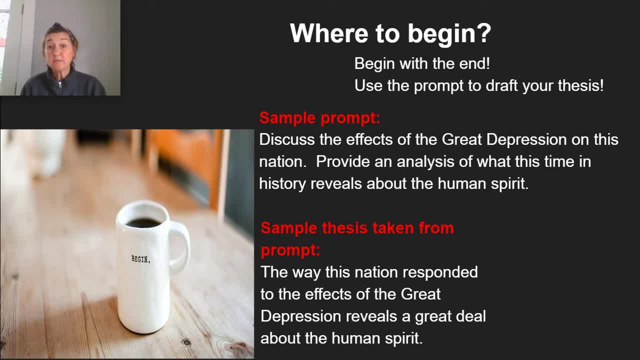 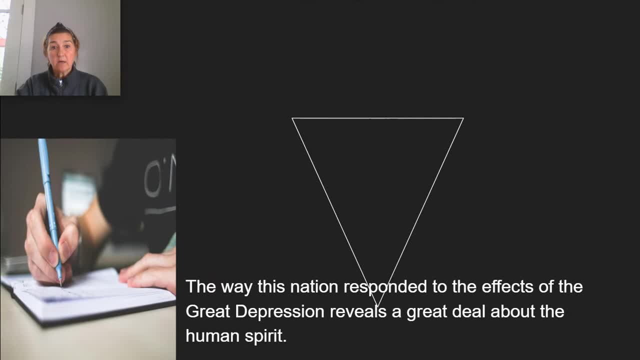 responses were: because I'm going to do that in my body paragraphs And I also didn't talk about what is revealed about the human spirit. yet Again, I'll wait for my body paragraphs to do that. So here we are. That's the bottom, That's the most specific. So now I got to go back and add: 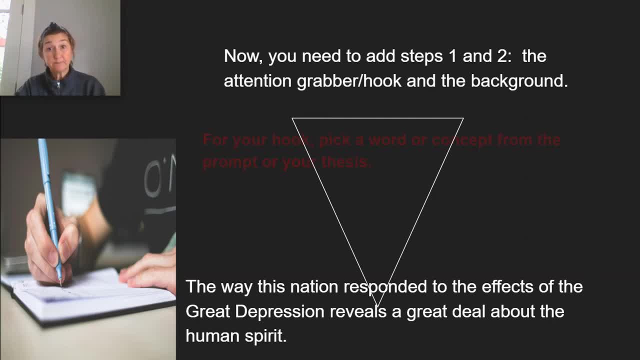 steps one and two, which is the attention grabber and the background. So what I always try to do for my hook is I look at the prompt, I look at my thesis and I try to find a word or a concept that I think is going to be really important. So when I think about the Great Depression, 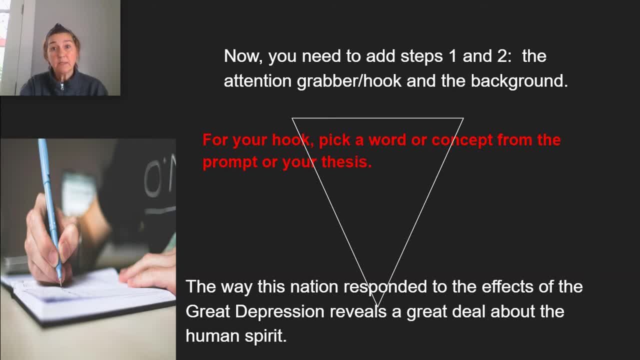 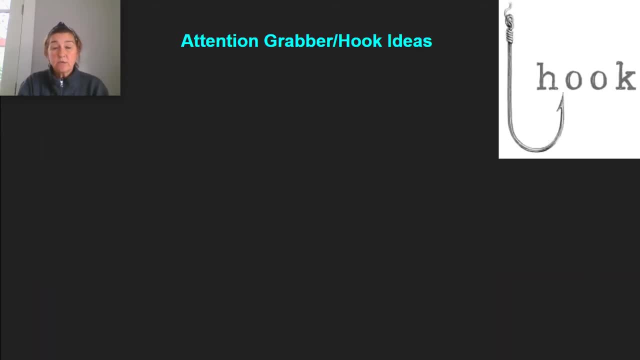 I think, ooh, that was like really challenging, hard time for a lot of people. So I'm going to start with something about challenge, because it's related to a concept that's in my thesis. There are a couple ways you 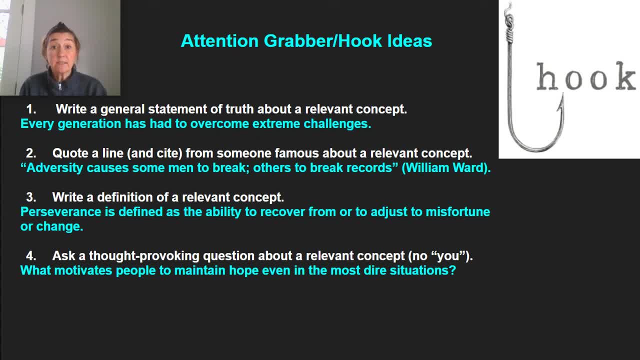 can do that, So you can write a general statement of truth about a relevant concept. So if I'm like, okay, the Great Depression is super challenging, I'm going to write a general statement about challenges. Every generation has had to overcome extreme challenges. I can also, if I want to. 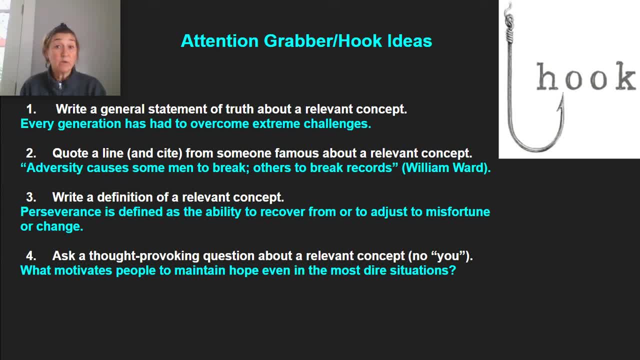 for my hook. instead of doing a general statement, I can actually find a line from someone famous about a relevant concept. So I literally Googled adversity quotes And this is what I found: Adversity causes some men to break others to break records, And that would be a nice way to open an essay. right, You can also write. 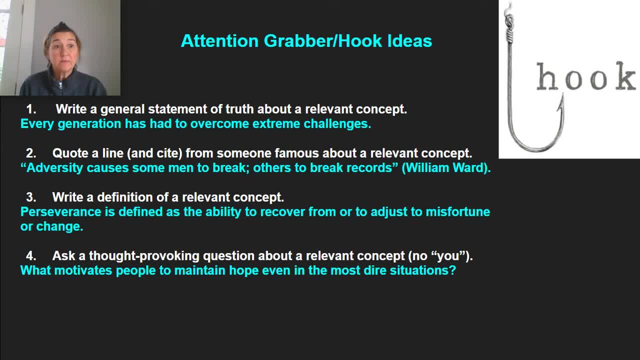 a definition about a concept that is relevant. So I literally looked up the definition of perseverance, because perseverance is something that people had to do during the Great Depression, So again, it's related or relevant. Perseverance is defined as the ability to recover from or to. 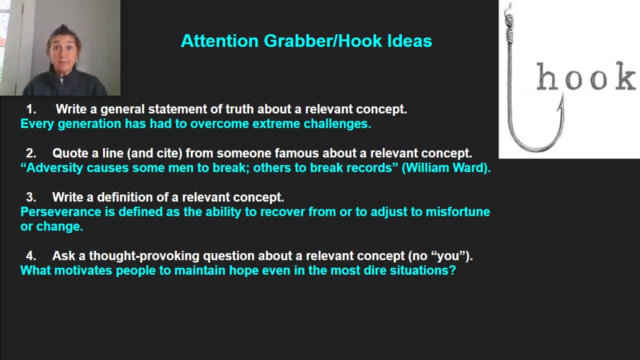 adjust to misfortune or change, And that's going to kind of set up that big idea. The last thing you can do is you can ask a question, but I do want to encourage you to avoid the word you, because it's too informal and it's too immature for secondary writers. So this is when I came up with 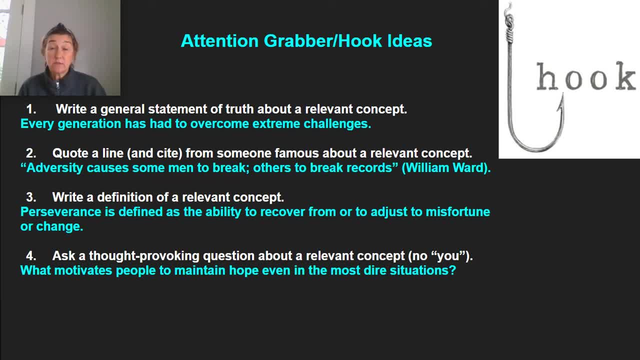 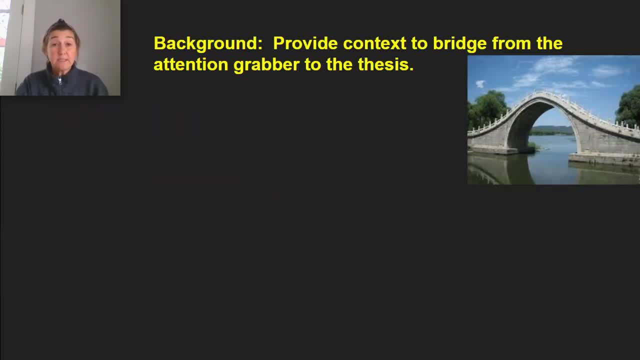 what motivates people to maintain hope in even the most dire situations, because the Great Depression was very dire, But yet there were people who maintained hope. The background step is step two, and it is the bridge between your attention grabber and your thesis, So depending. 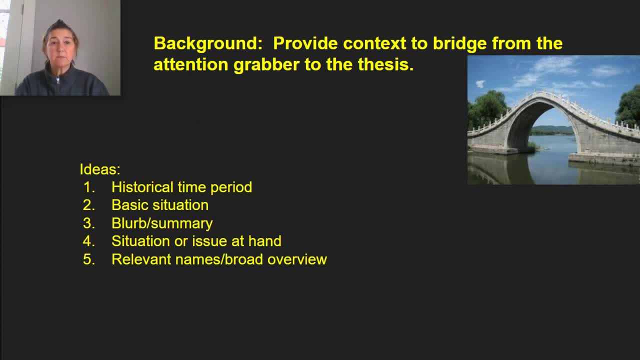 on what your prompt is. sometimes you have to give a little history context. Sometimes, if it's about, you need to write a little summary with a title and author about the piece, to remind readers what that piece was about. It's an argumentative paper. You might want to explain the issue at hand and 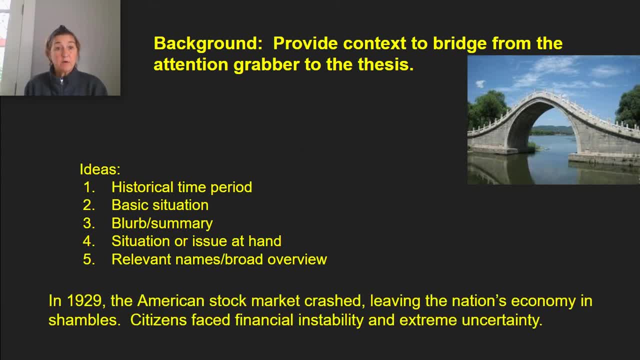 the two sides that people argue about. So here's what I came up with for ours. In 1929, the American stock market crashed, leaving the nation's economy in shambles. Citizens faced financial instability and extreme uncertainty. So giving a little context so the reader knows: oh okay, I remember. 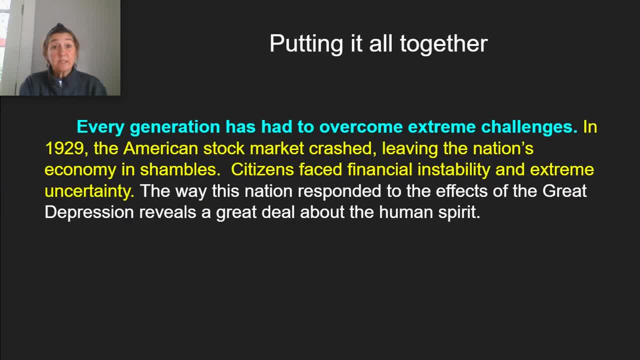 what was happening during that time, And then the only step left is putting it all together. So you can see that you have these three steps. It's four sentences total. You could write a little more, You could write a little less. You just want to make sure that you have all three of those. 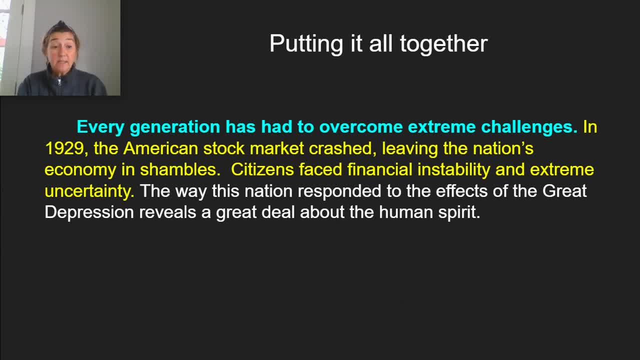 steps, And that's it. So hopefully this was helpful. You're always welcome to, of course, watch them again, But if you have other needs, go ahead and check out my YouTube channel and see if there's something there that will help you. Hope to see you again soon.